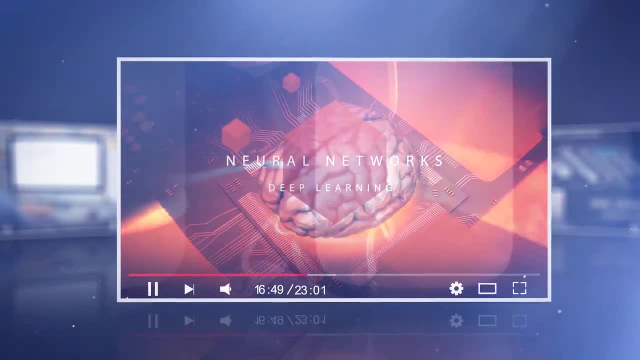 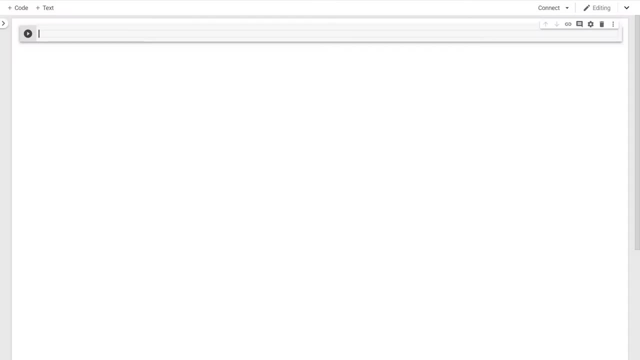 Hello guys, as we all know, the success of any machine learning model is dependent on the data that is being used to train. So the way we split the data has a direct impact on the accuracy we achieve from our model. Hence, it is very important that we know everything. 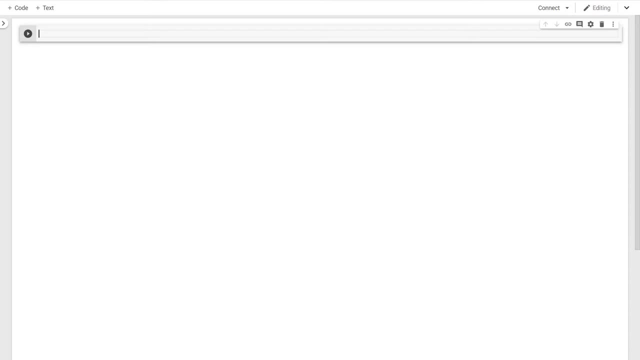 about the function we are using to perform the split, And one of the common functions we use to perform the split on the dataset is trainTestSplit function, which comes under sklearnmodelSelection. So, guys, without wasting much of time, let's get started Here. as a first step, I'll start by importing. 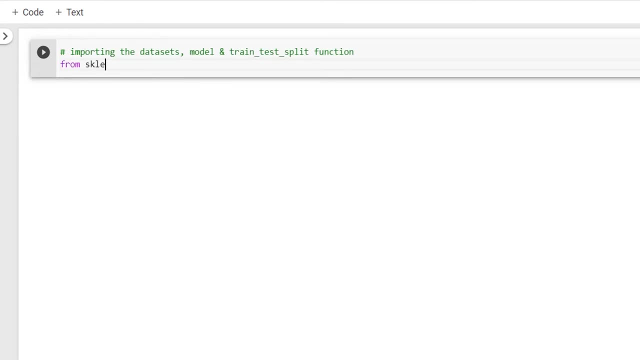 the dataset's model and trainTestSplit function. So I'll write as: FROM sklearn: import datasets- linear model And then FROM sklearnmodelSelection: import- trainTestSplit. So now here in this video I'll be using the diabetes dataset which is available inside. 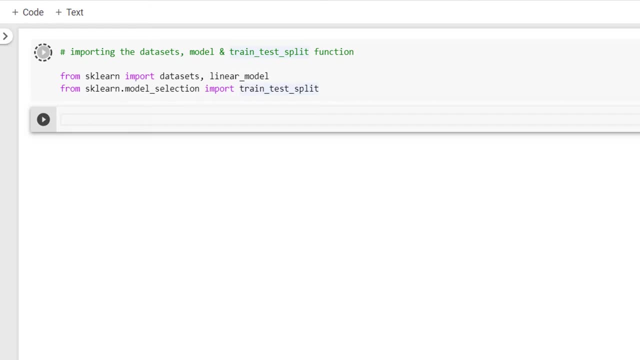 the sklearn library. So I'll load the dataset like this. That is, diabetes is equal to datasetsloadDiabetes, So this will load the dataset And after that I'll separate the input and output, as x is equal to diabetesdata and y is equal to diabetestarget. 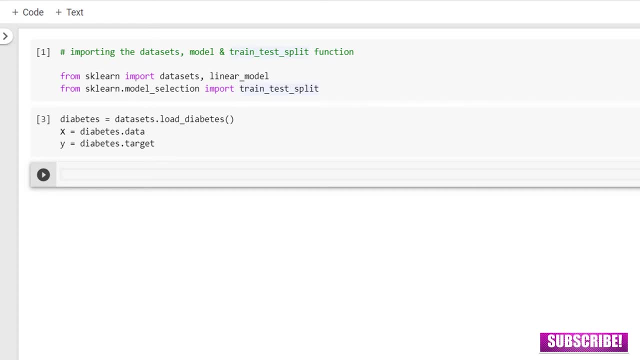 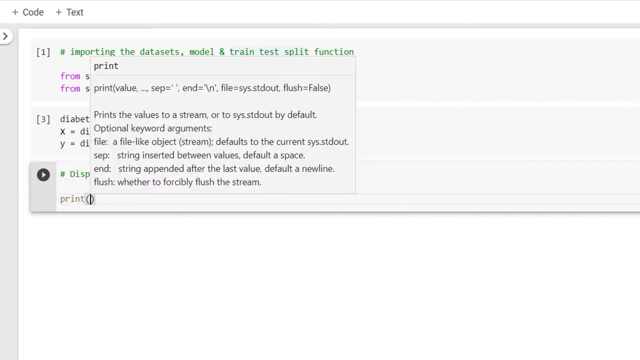 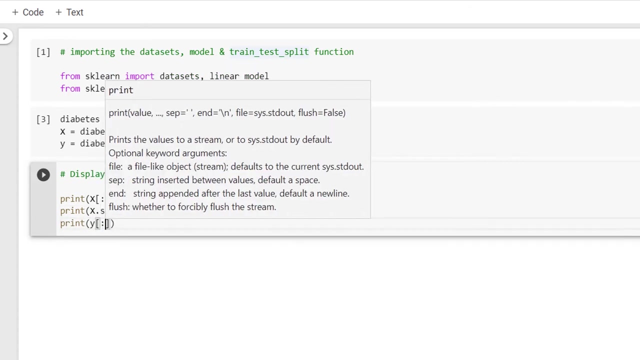 Ok, we have now loaded the dataset for our working. So now let's display the shape and first few elements in our data. So for that, print x colon phi and then print x dot shape. And for this y, print y colon phi and then print y dot shape. 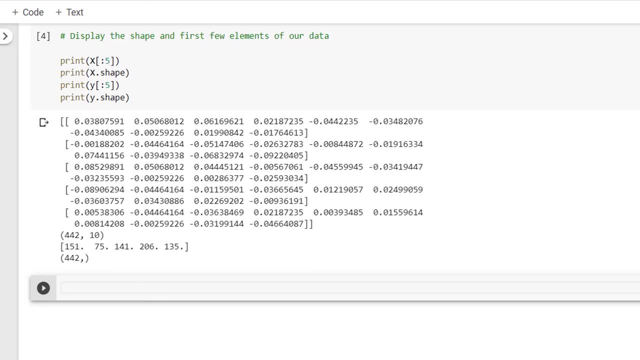 Okay, we have the input data x of shape 442 comma 10.. That means we have a total of 442 rows and with 10 features for each row, And then target y is of shape 442.. That means it's a single dimensional array. 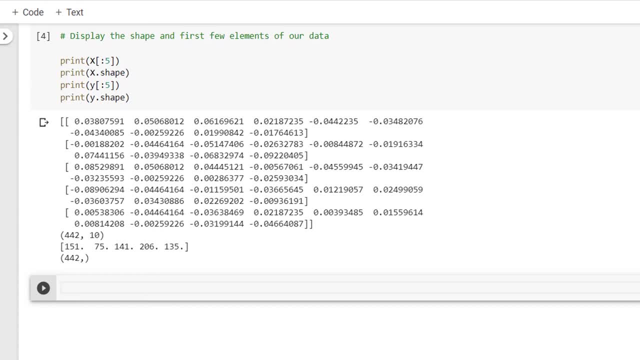 And here, if you observe the values that array y contains, is the real values. So I can say: as this is a regression task, Now the next step is split the data into two parts, That is, training data and validation data. So for that we are going to make use of train test split function. 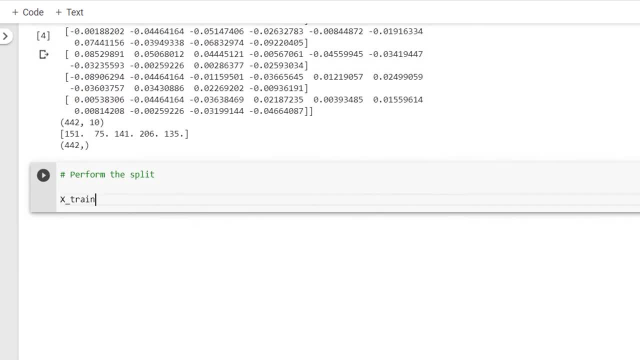 And to perform this split we can call the function like this, That is, train comma xtest comma ytrain comma ytest is equal to train test split of x comma y. Okay, this has been executed. So now let's display the shape of xtrain, xtest, ytrain and ytest. 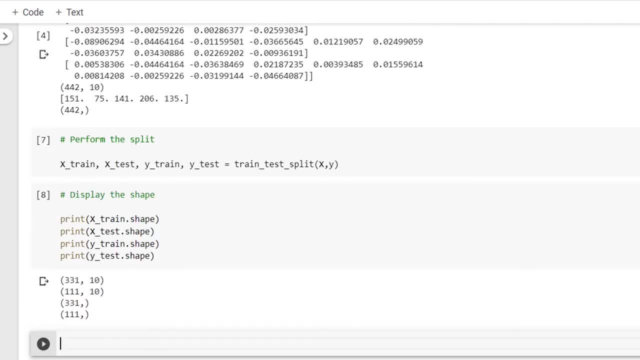 Yes, as we can see from the resulting shapes of arrays. that is, we have splitted the training data and test data in the ratio of 7.. 70 is to 30. That means 70% of data are splitted as training data and the remaining 30% are the test data. 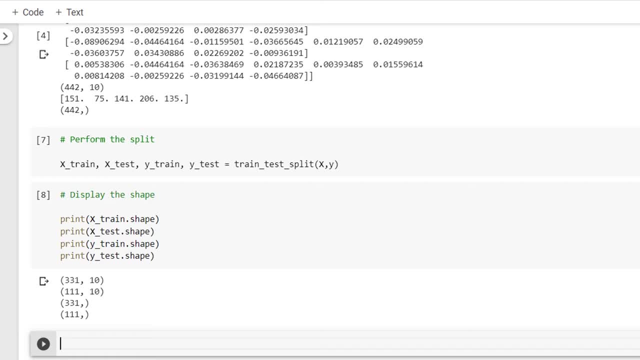 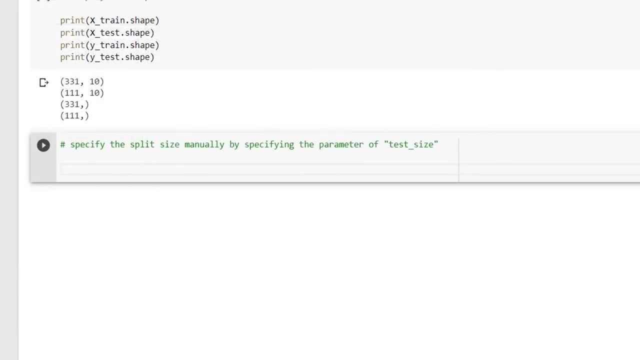 Now, if we want to specify the split size, then we can do it manually by specifying the parameter of test size. So to show you how it is done this time I'll perform the split like this, That is: xtrain comma, xtest comma, ytrain comma- ytest is equal to training data. 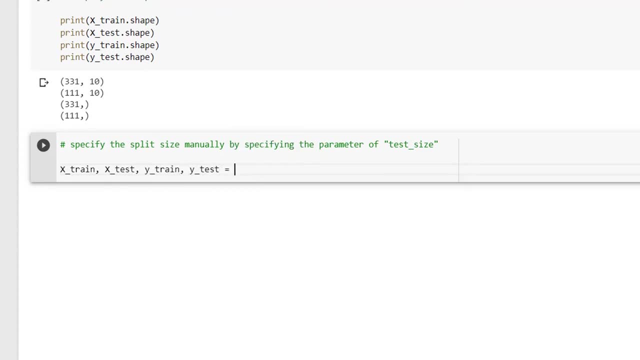 So now I can specify the split size. So I can specify the split size And then I can specify the split size. By doing this, we can see here that the split size is equal to training test. split of x comma, y comma test size is equal to 0.1. 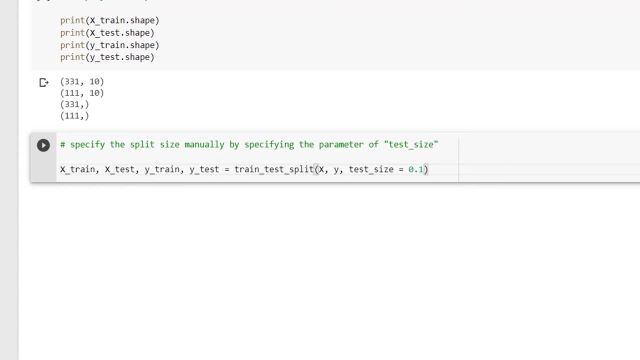 As you can see here, this time I have specified the test size as 0.1. That means only 10% of data will be used as test data and the remaining 90% will be used as training data. So let's confirm it by printing the shapes as well. 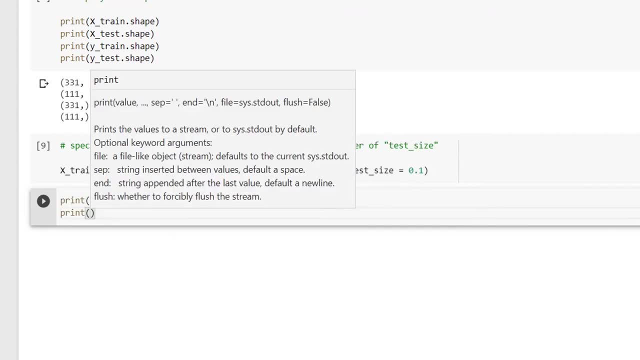 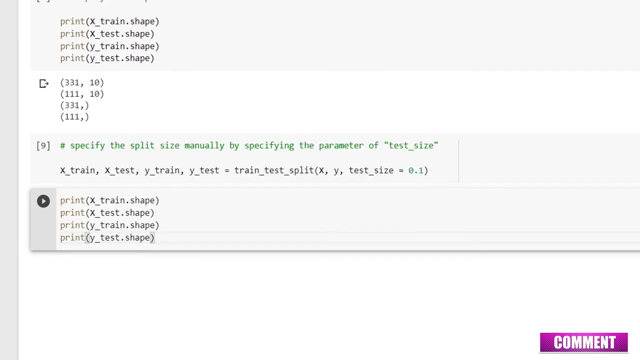 xtrain comma. ytrain test split is equal to training test split and the remaining 90% will be used as training data. that is, print x train dot shape and then print x test dot shape, print y train dot shape and print y test dot shape. as we can see from the output that we can observe that the training data 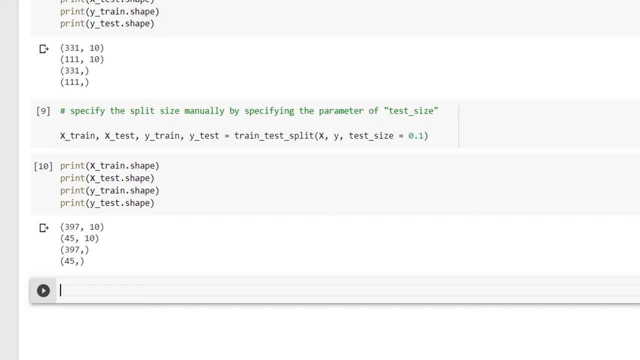 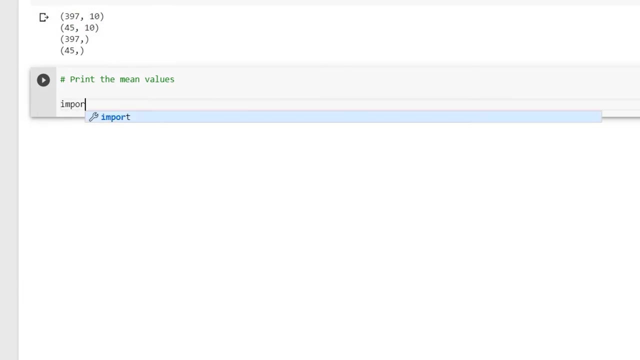 now has 397 rows and the test data has 45 rows. so in this way we specify the split ratio when using the train to split function. okay, so now let me print the mean of the values from the data set, for that it will be like import numpy as np and then print np dot- mean of extreme. then 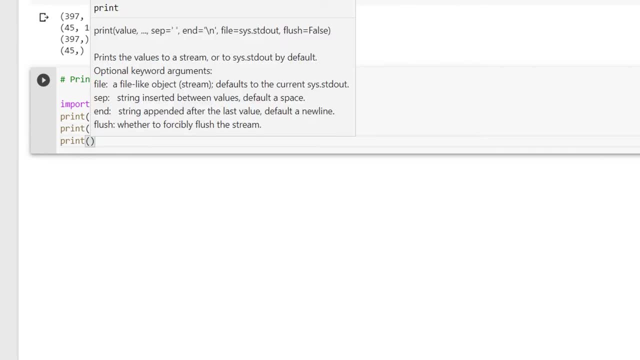 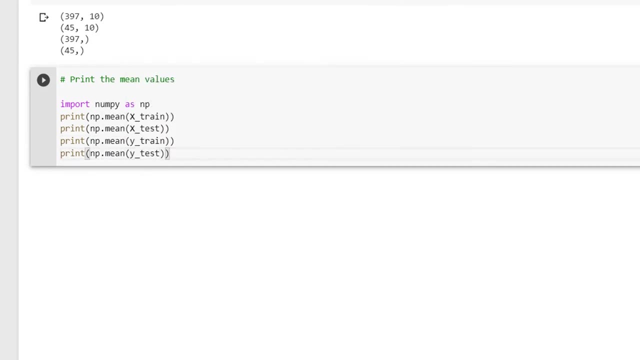 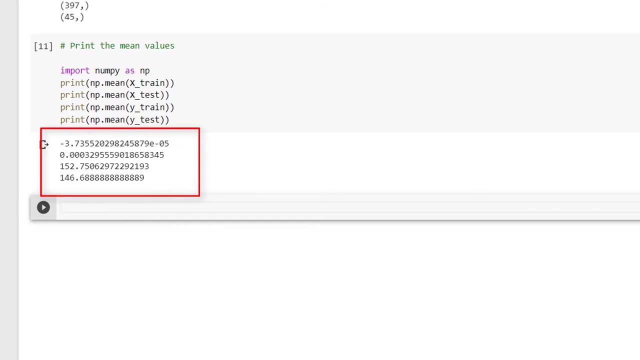 print np dot mean of x test, and after that it will be like: print np dot mean of y train and print np dot- mean of y test. as you can observe, that is like we have the mean values of the training and test data like this. now, what i'll do is i'll 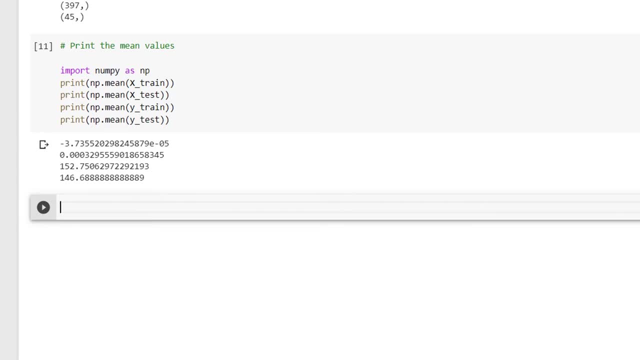 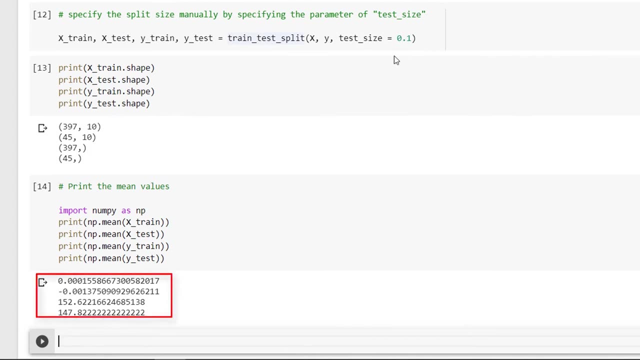 again run the train test split function and then compute the mean. okay, as we can observe here, that is, each time when i run a split function the mean values are different. that means a separate split of data is created each time the function is run now to be able to get the same. 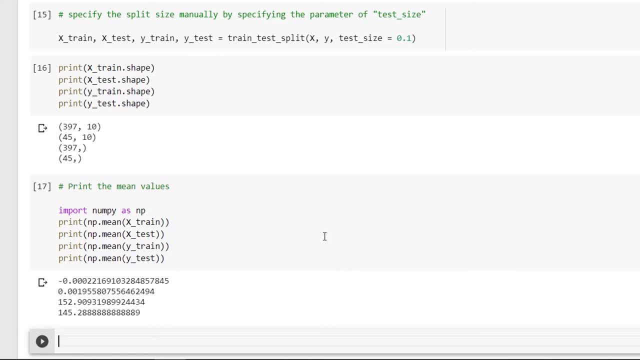 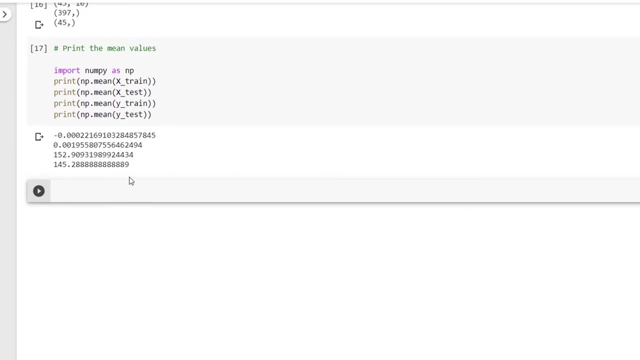 split. every time we have to specify the random state instance with the use of the parameter random state, that is, random goes state. so this time i'll write as extreme: comma x test, comma y, train comma y test is equal to train test split off x, comma y, comma test. 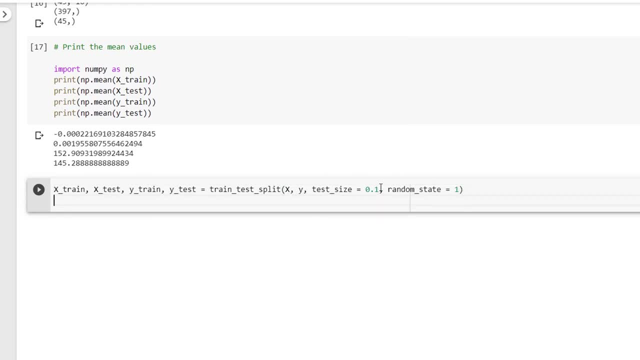 size is equal to 0.1 comma, random state is equal to 1, and then i'll execute the code. okay, this has been x test and spj test. multiple types of spj will not aroma, and also also between the far left camper way to go tofon. to our screen, as well as the j appears chша's NYU base an富 system of long space with the text 여, i, 0,, 1 and, of course, if we 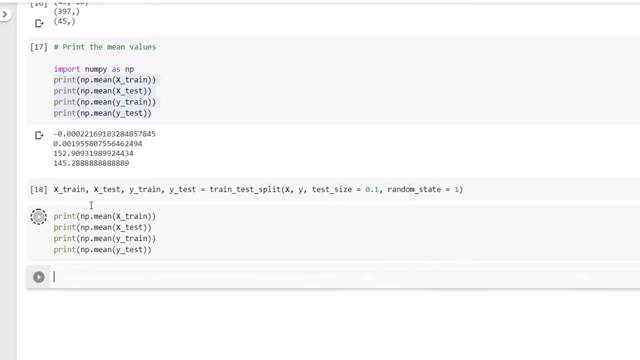 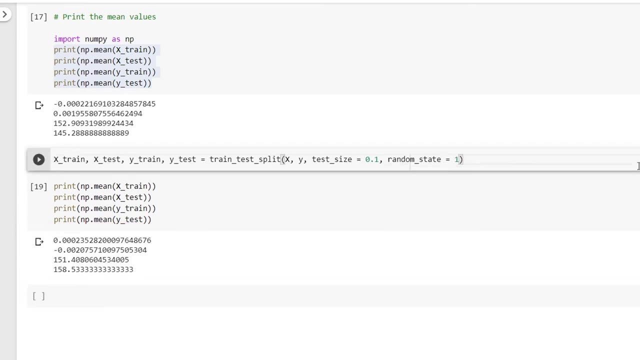 execute it and i'll now compute the mean. okay, we have the mean values like this, and this time i'll again perform the split function and see what happens to the mean of the data set. all right, as we can observe here. that is no matter how many times i run the code. 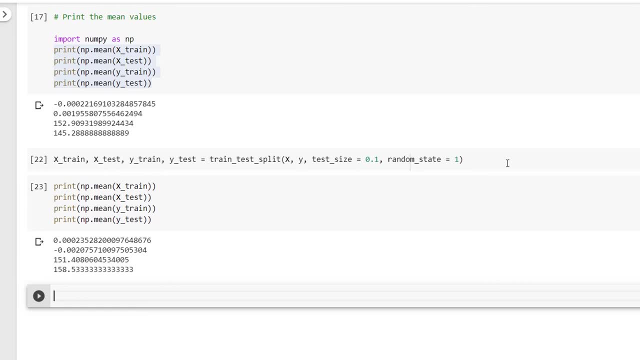 the mean is still the same. that means each time, each time, we get the same split on the data and if you're using a classification data set, then you can also make use of the parameter stratify. yes, you can use this parameter stratify to get the stratified split. so, guys, i hope 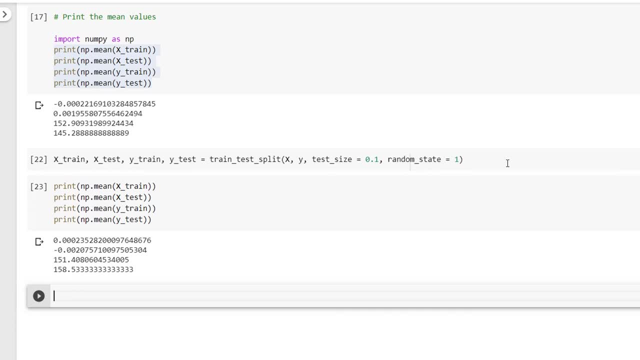 you now know as how to make use of the train test split function to efficiently split the data set, and i'll see you next time. you.